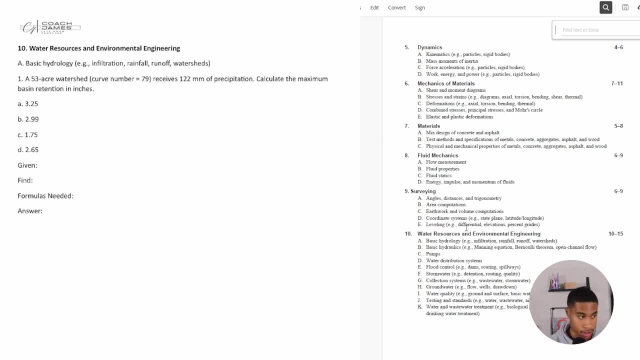 All right. so number one says a 53 acre watershed, the curve number equal to 79, receives 122 milliliters millimeters of precipitation. All right, Calculate the maximum basin retention in inches. So what is? what is the information that I'm given given? 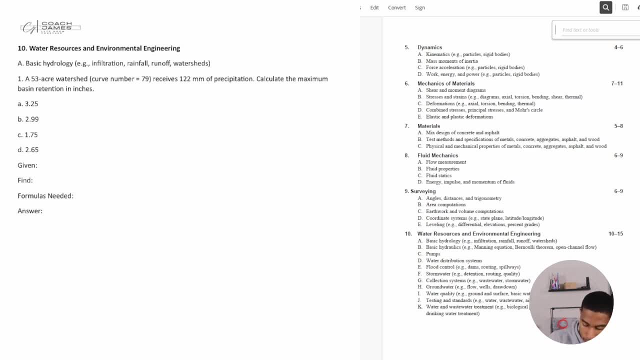 some get a green for passing. So, given information is we have our curve number of 79, right. We are also given that the amount of precipitation is precipitation And we're also given the area, Okay, And so calculate the max. So we're trying to find the max. 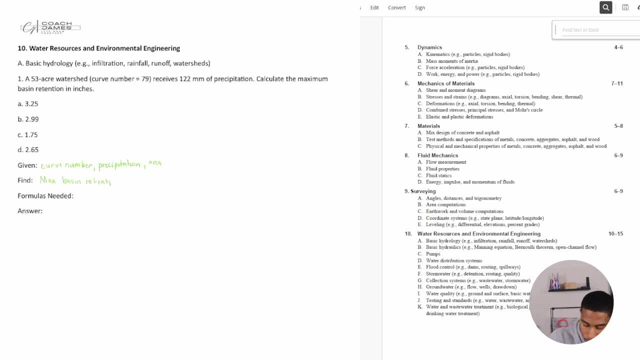 basin retention. Okay, And it should be in inches, All right. All right, So I'm just going to look up- I don't know what formulas I need to use- for this is a bunch of random data for me- that it's going to look up what I'm trying to find, which is basin retention. 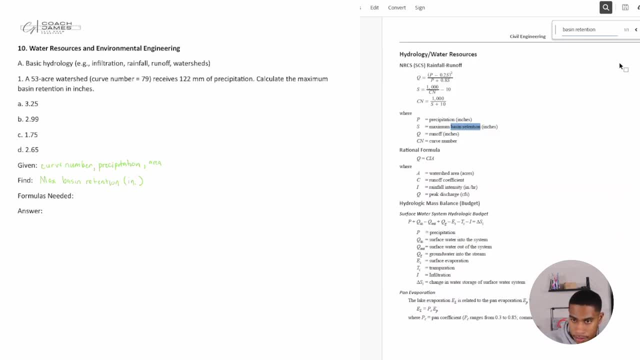 One thing comes up And okay, S is equal to maximum basin retention in inches. Okay, Basin retention in inches. Cool, So I feel like I may be in the right area. It's the only thing that search as well, So S. 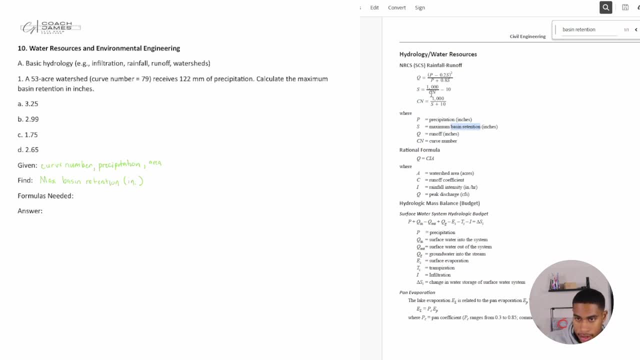 So S is equal to, okay, 1000 over CN minus 10.. CN is our curve, is a curve number and we have a curve number which is 79.. So I have all the variables. I need to be able to solve this question. 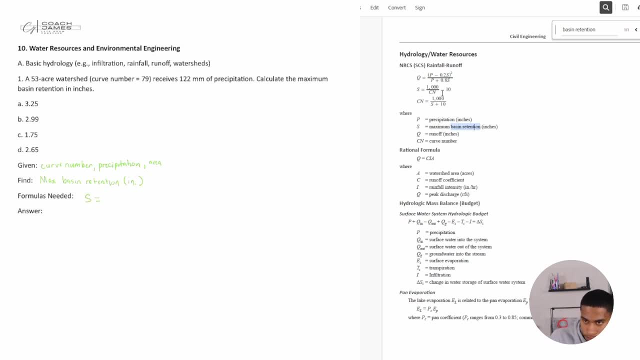 So I'm going to say S is equal to 1000.. Over the curve number Minus 10.. My curve number is equal to 79.. So This is all going to be equal to 1000.. Over 79.. 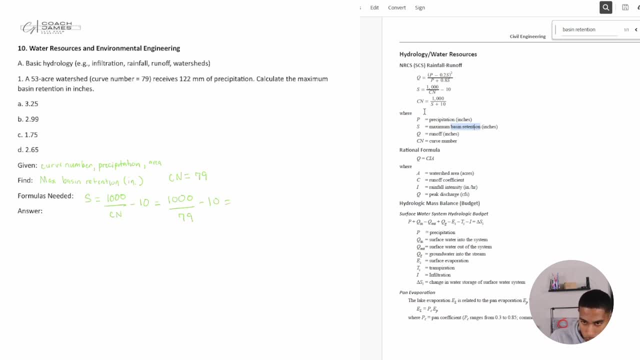 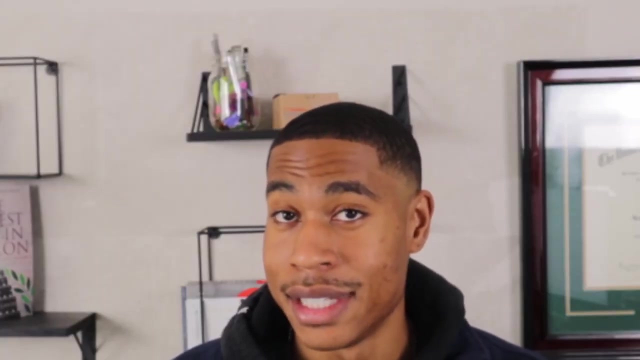 Minus 10.. And so S The maximum basin retention In inches is going to be 2.65 inches. So I get D. Hey everybody, I know I didn't take time to formally introduce myself at the beginning, So I did want to let you know who I am and how I can best serve you as you're studying for your civil F E exam. 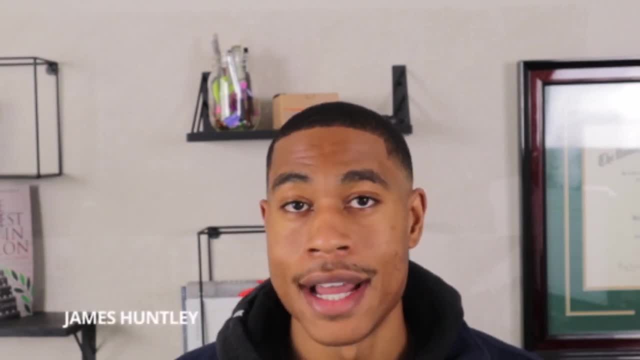 So my name is James Huntley And I am a civil engineer Who has helped hundreds of individuals pass and dominate their civil F E exam. Now I know this test is tough And as you're going through material, you may be saying: 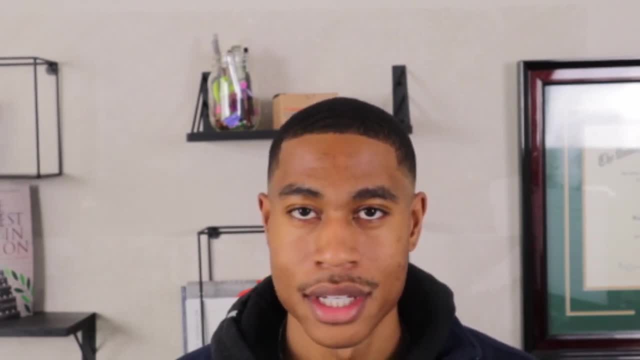 I don't remember learning this stuff, or Gosh, these variables are so confusing or you just feel like you're really, really busy And there's so much material that you need to go through That it's a bit overwhelming. So 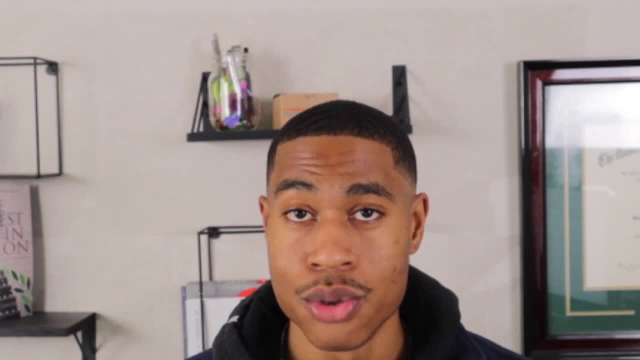 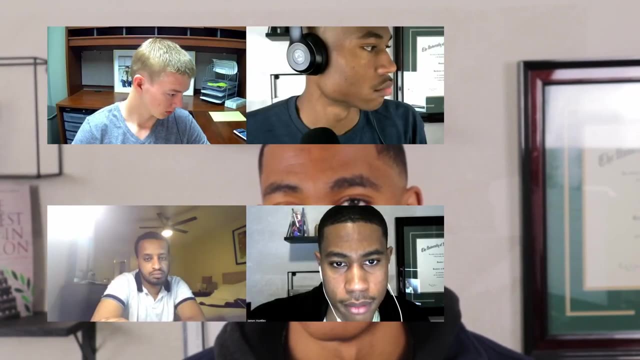 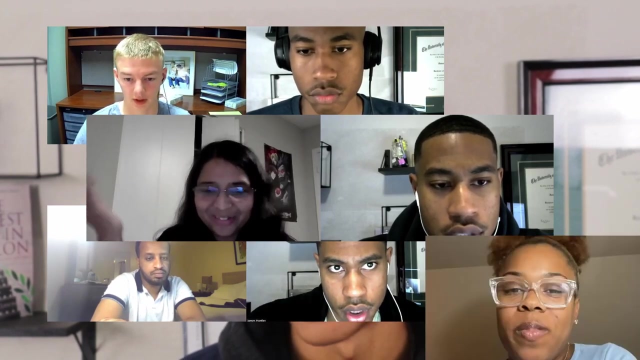 Did want to let you know that I do help and work with individuals one on one To ensure that they pass their civil F E exam, And I've had individuals that have worked with me for 10 weeks And that's the longest that has been. 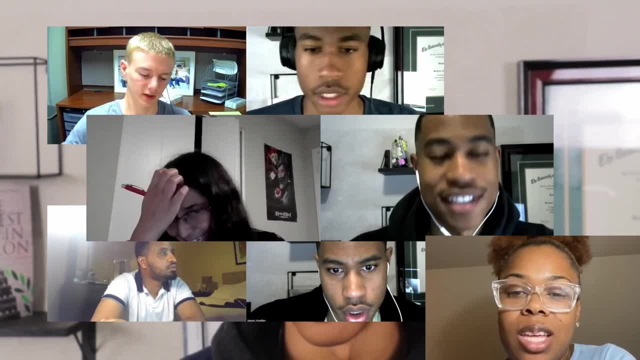 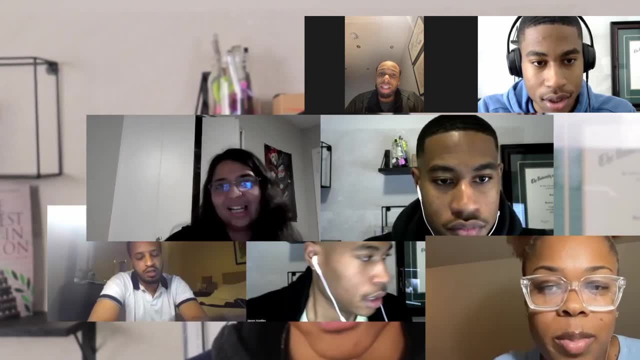 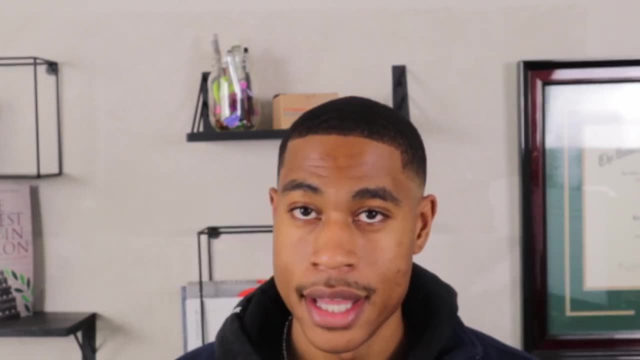 And I've had individuals that have worked with me for two weeks And we went back to back day after day after day, Hours on hours, on hours, Putting in the work, Working together to ensure that they went ahead and passed Right. And this exam is so important because I know that you want to make more money. 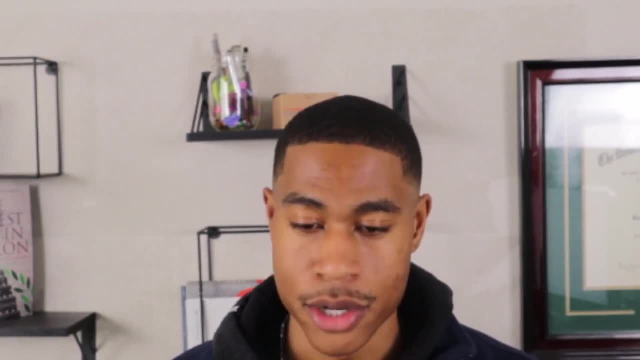 I know that you want to, you know, get some promotions And be able to further your career and have your P? E. So definitely want to open and extend a handout, Want to be able to save you time, Right, Because I know some people that watch my videos. 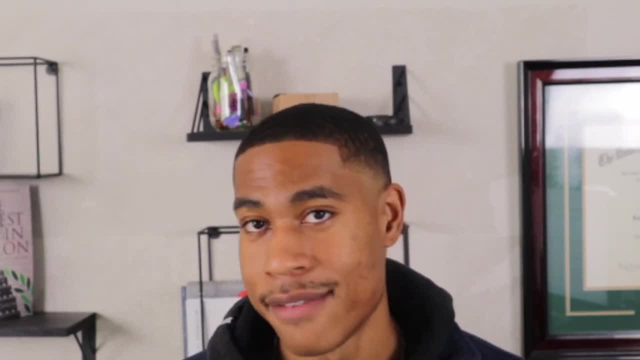 You may have been watching my videos for six, Nine, Even 12 months And you still haven't passed your civil F E exam, And that is the one thing that's keeping you from making more income or impact And furthering your career. 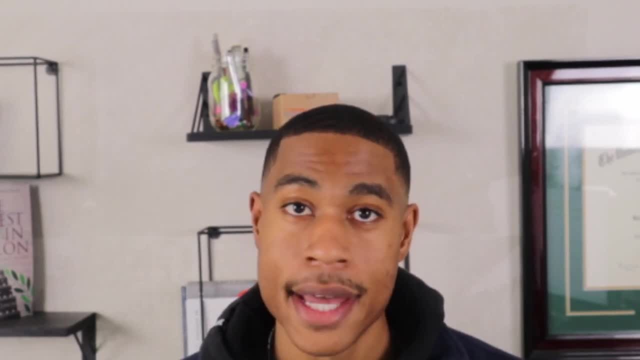 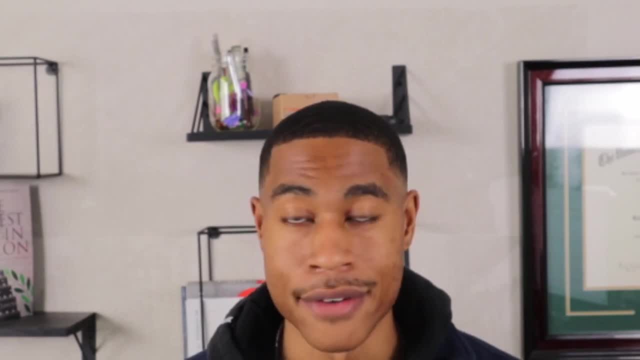 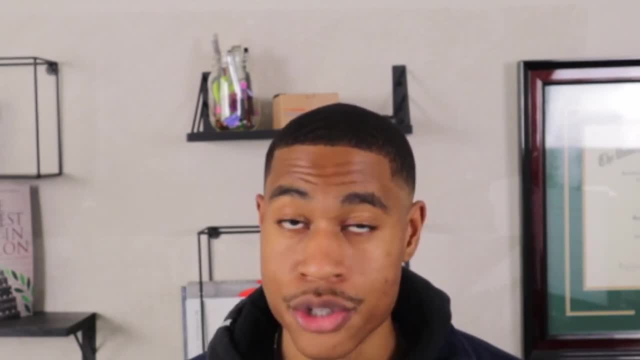 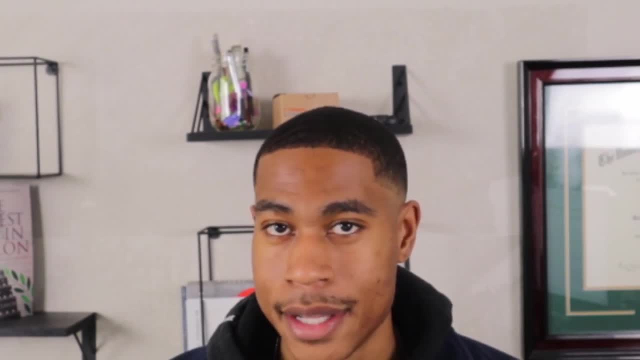 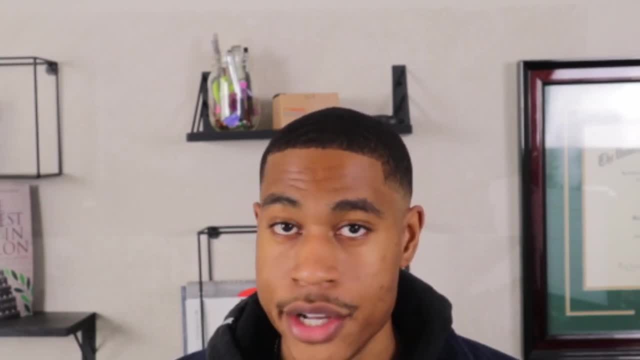 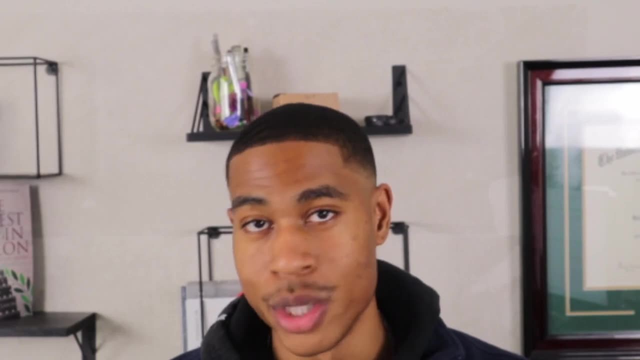 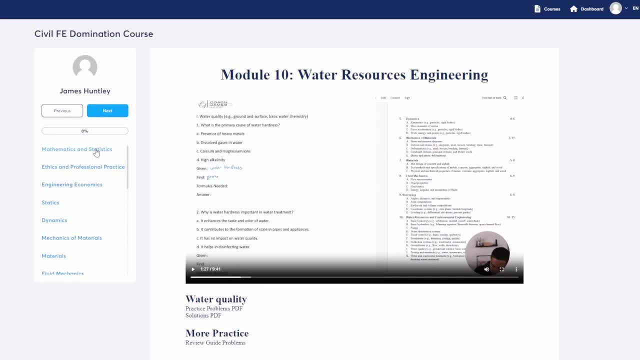 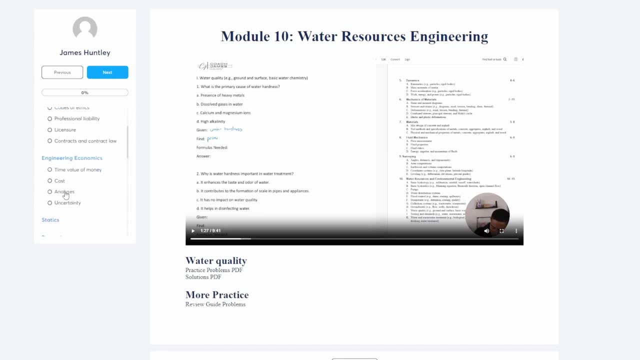 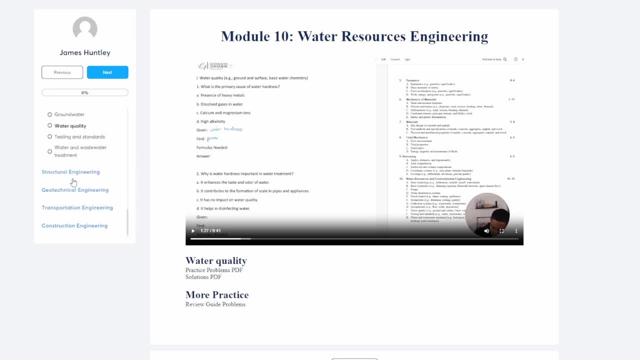 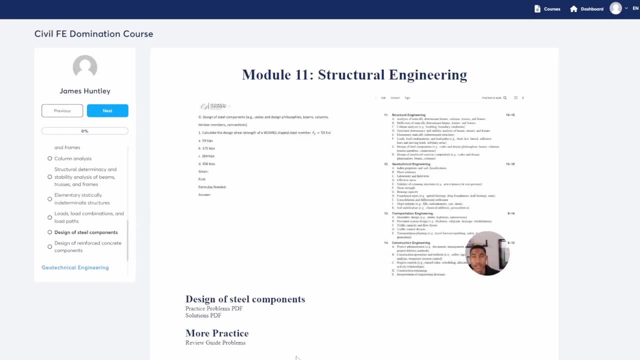 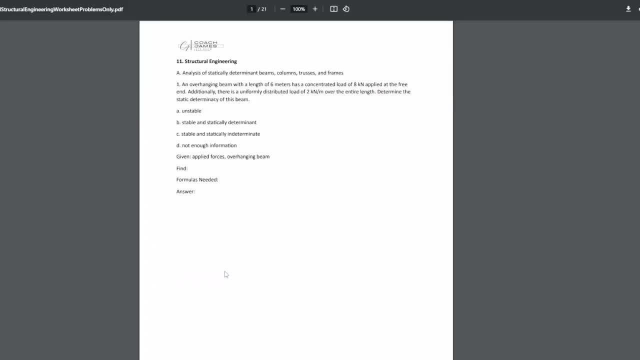 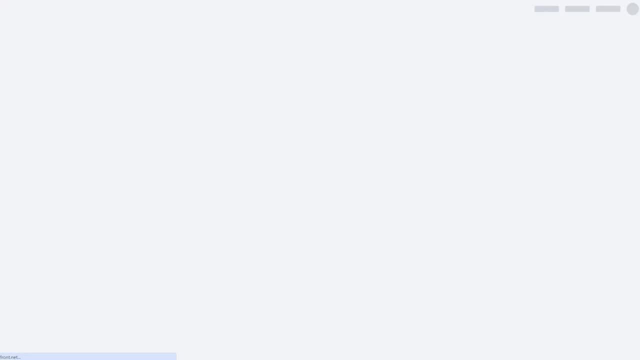 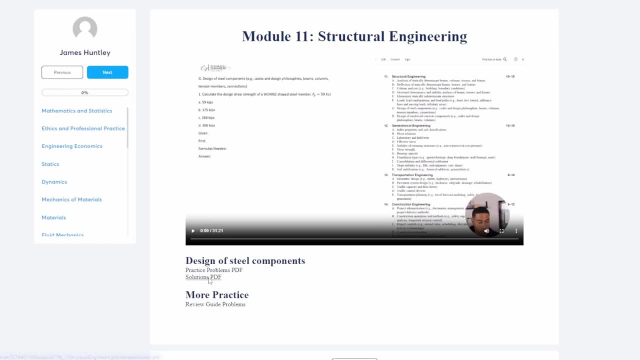 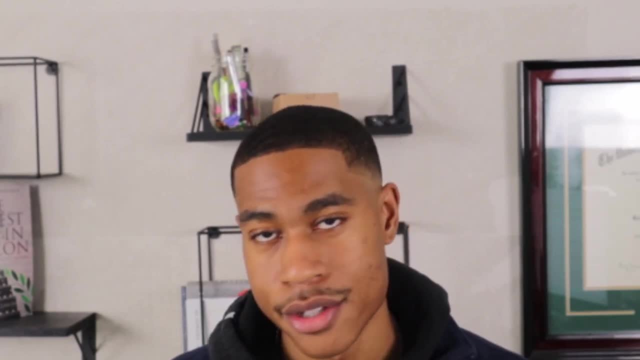 So It's definitely costing you Money resources everything. So It's definitely costing you Money resources everything. So It's definitely costing you Money resources everything. So Down in the description box below I have a ton of resources, including one-on-one coaching. 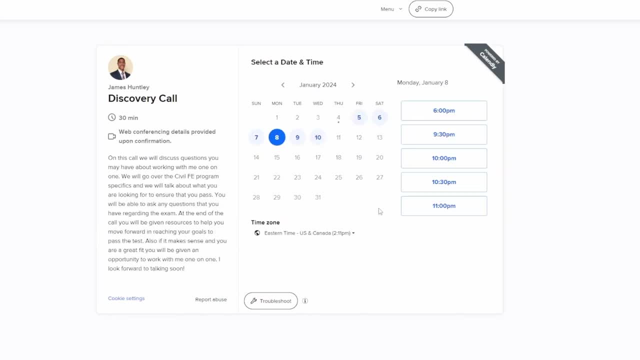 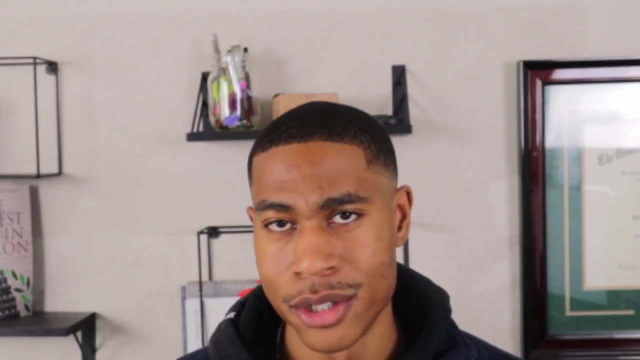 Just hop on a call. It's no cost to you as far as you know us talking through your goals and what you're trying to do and kind of getting a feel for where you're at. So I have some programs where I can work with you one-on-one.